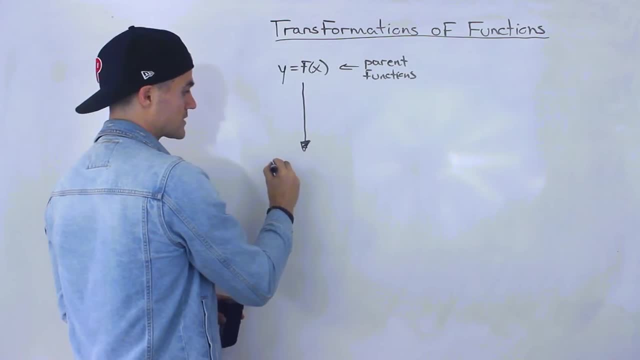 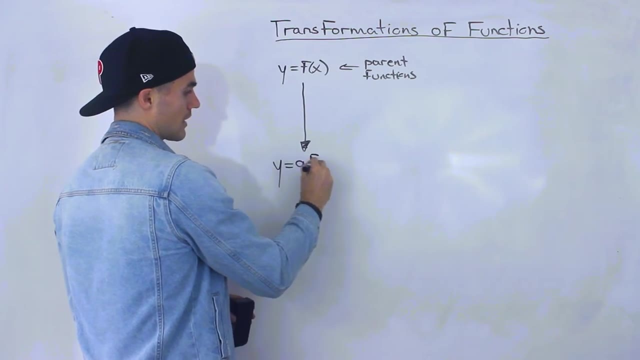 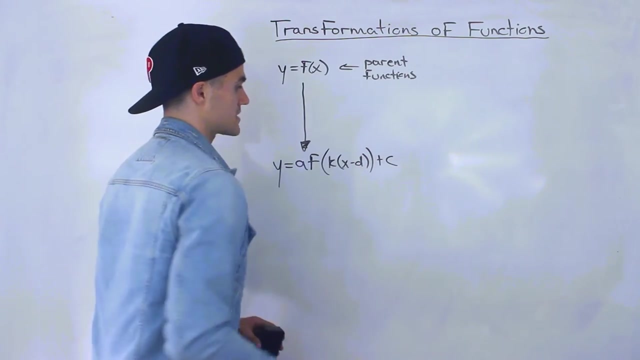 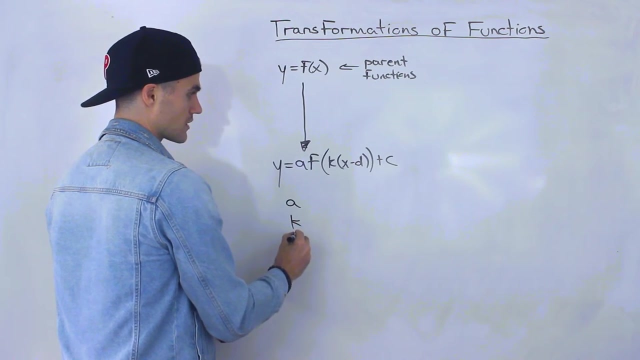 with here. but just in general, you can take a function and when you transform it it's going to take this value, this expression here, this format, rather sorry, a f of k bracket, x minus d plus c, right. So notice that we added a bunch of letters here. 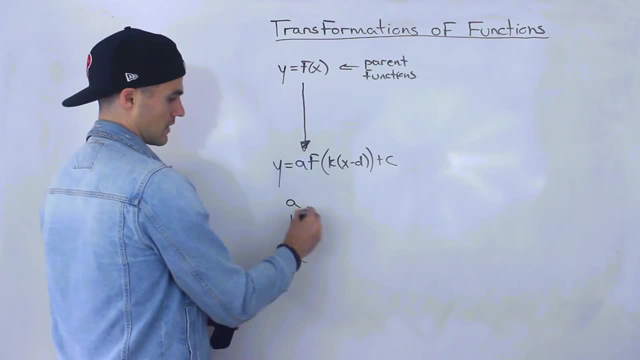 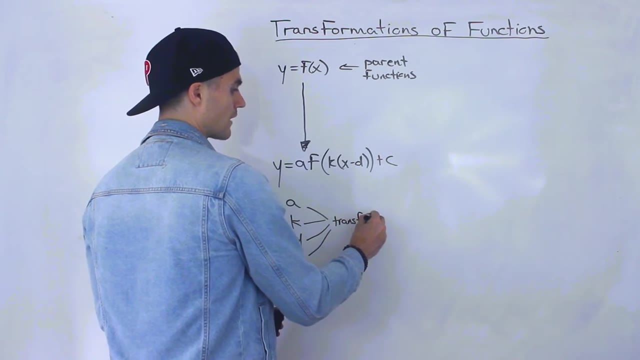 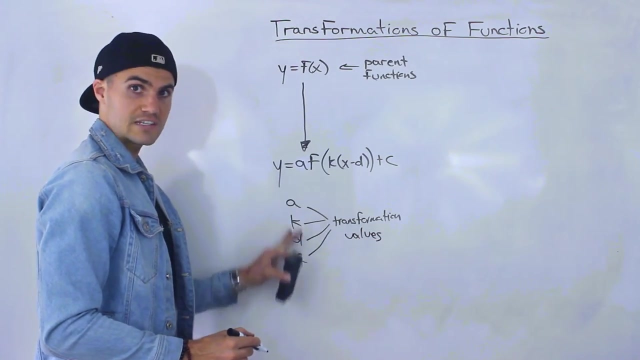 a, f of k bracket, x minus d plus c, right? So notice that we added a bunch of letters here- K, D and C- And what I'm going to refer to these, as throughout these videos, is the transformation values. Okay, so the values of these letters here is going to tell you what type of transformations. 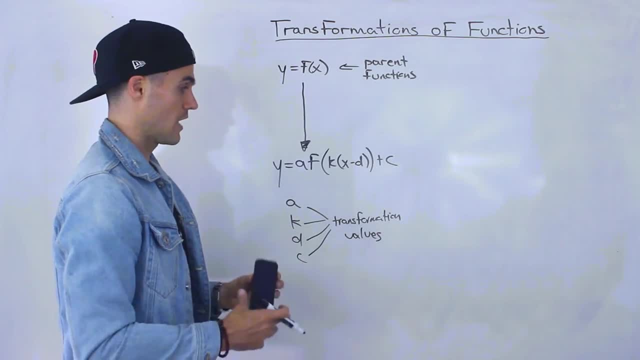 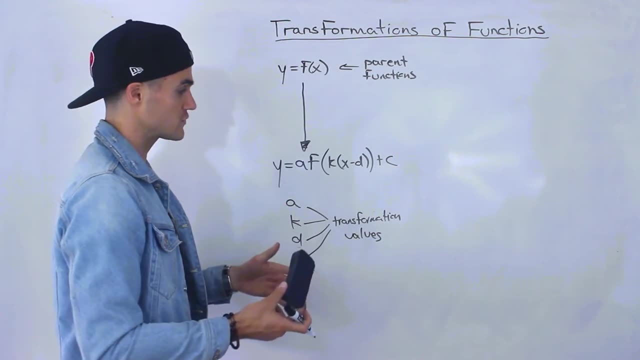 that parent function is going to undergo, And we're going to go over in detail in the next couple of videos what each of these specifically mean in terms of transformations. But just in general, that's what's going to happen. You're going to have a function like this, and then 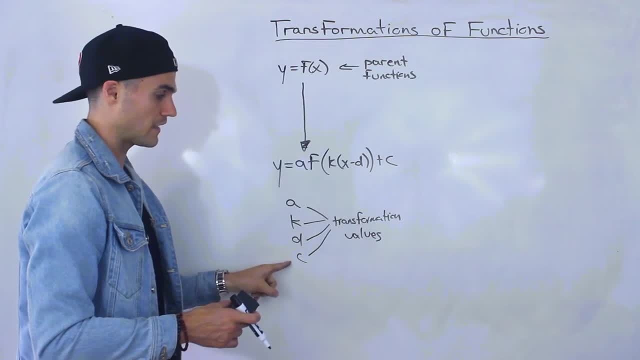 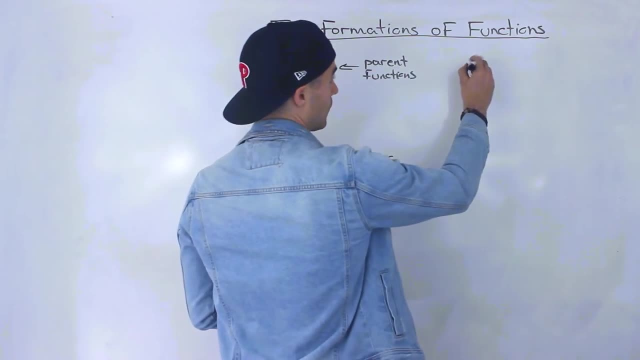 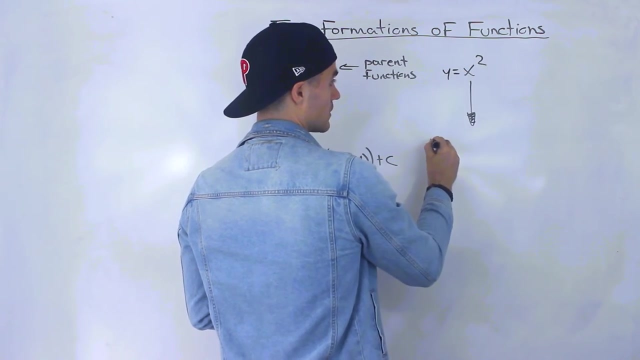 it's going to have all of these transformation values And, depending on what they are, the function is going to transform in different ways. So, for example, let's say that we have the parent function x squared, And now what we're going to do- we got y equals x squared- is we're going to transform it. So 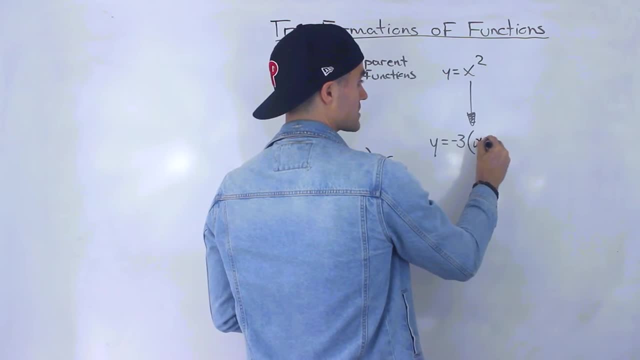 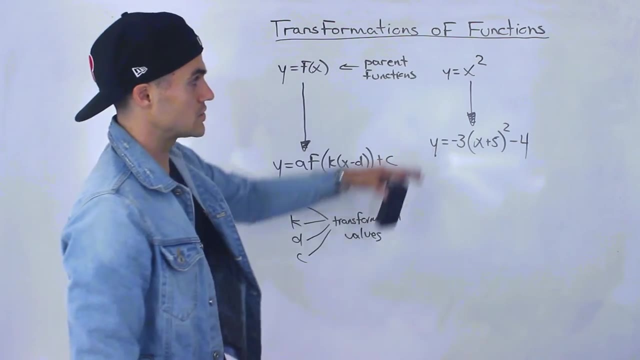 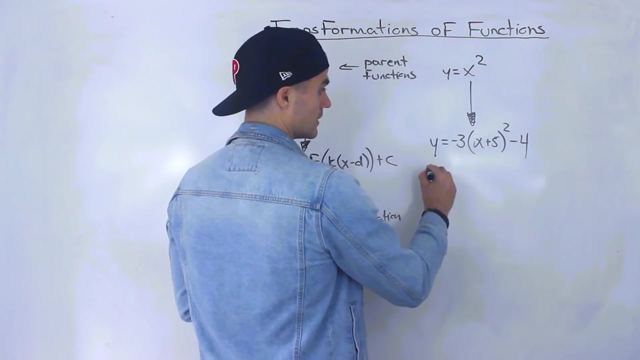 let's say we have a negative three x plus five squared, let's say minus four, right? So we took this x squared and transformed it a bunch. So basically, what's the a, what's the k, what's the d and what's the c value? 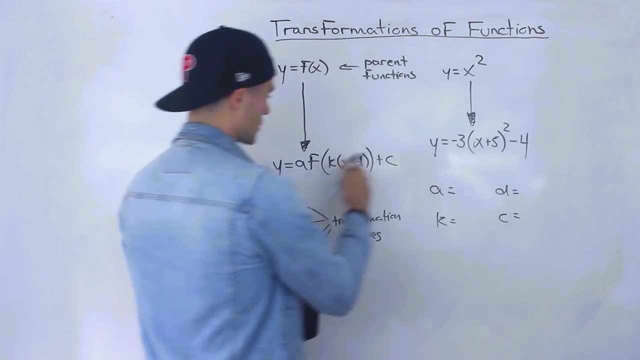 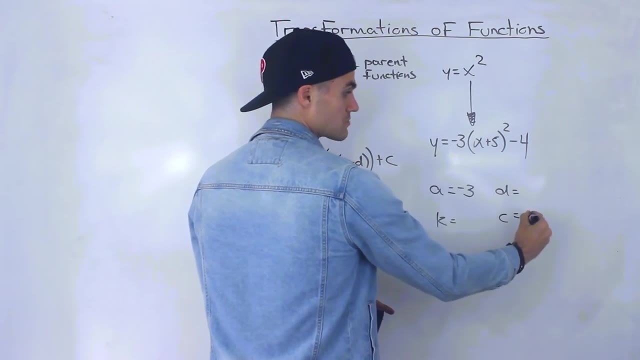 going to be here. Well, notice that the a value is always sort of on the outside, so it's this negative three, and then the c value is on the outside on this side here, so it's minus four. Those are usually the easiest ones to get. It's usually the k and the d value that can get a. 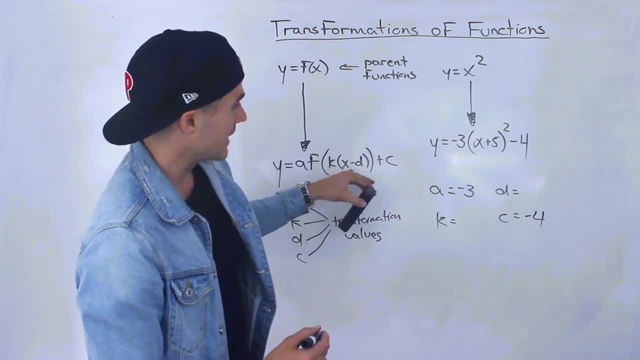 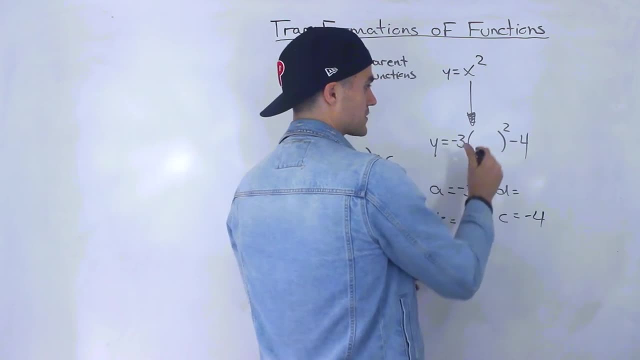 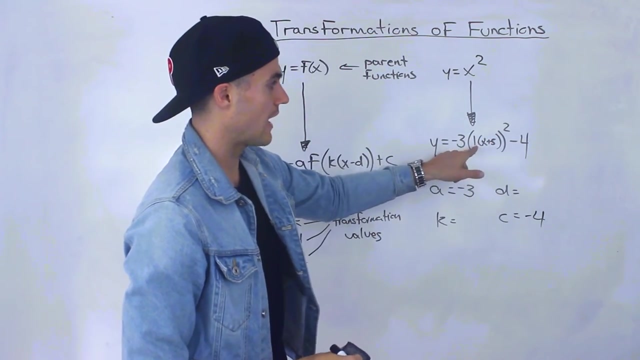 little tricky. So notice that we have k bracket x minus d. So notice that there's nothing in front here. So we can rewrite this x plus five as one bracket x plus five, like that right: x plus five and one bracket x plus five. 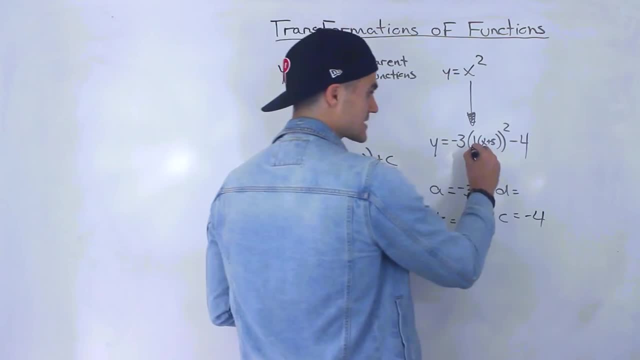 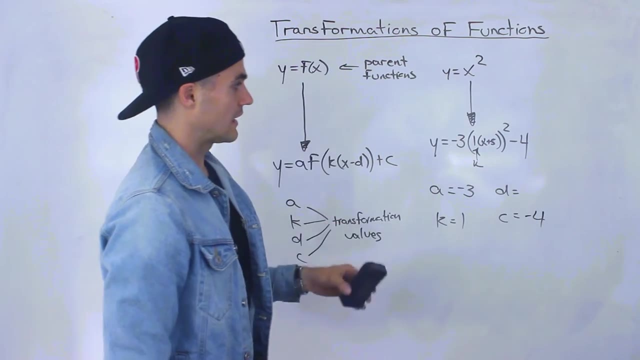 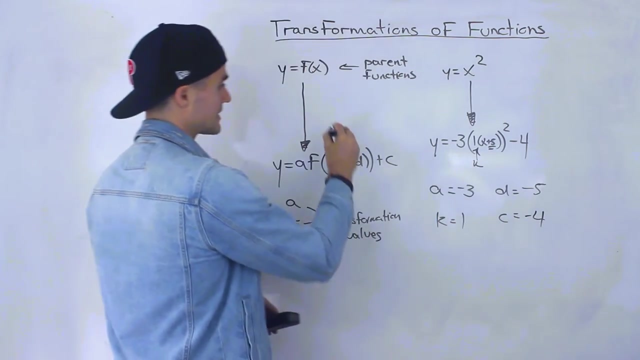 Those are the exact same thing, and the reason why I put it in that format is because now we could see the k value is one. What's the d value? Now, the d value is negative five. It's always going to be the opposite sign here, because- notice that it's x minus d. So if we have x plus five, 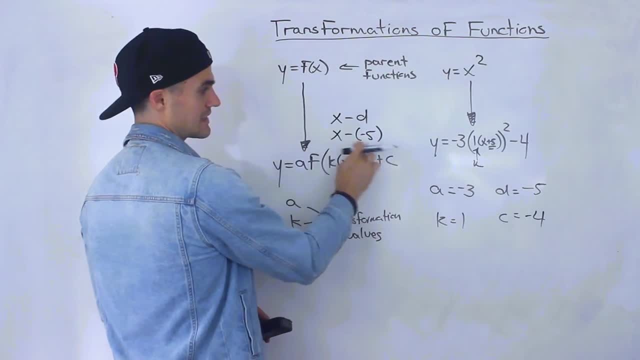 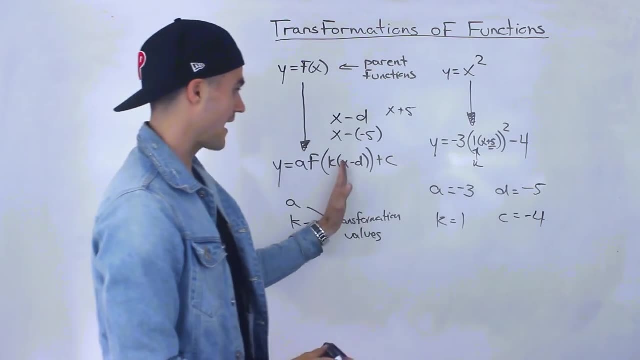 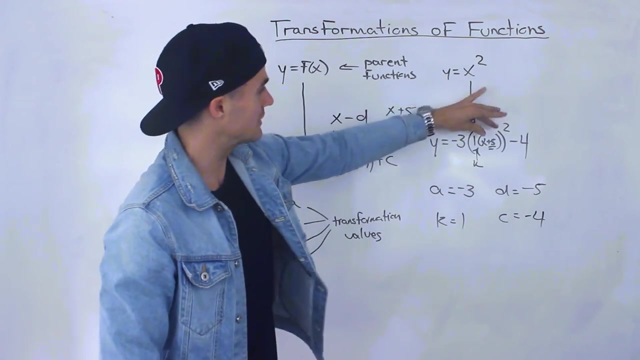 that's the same as x minus negative five. Notice that that is going to be x plus five, And so that d value is actually negative: five x minus d, x minus negative five, which ends up being x plus five. So whenever you have something like this, you got to kind of rewrite it like: 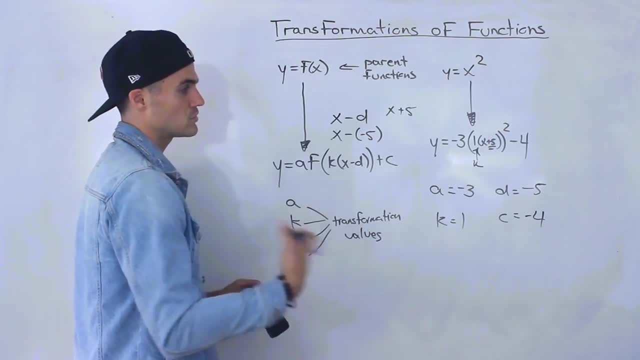 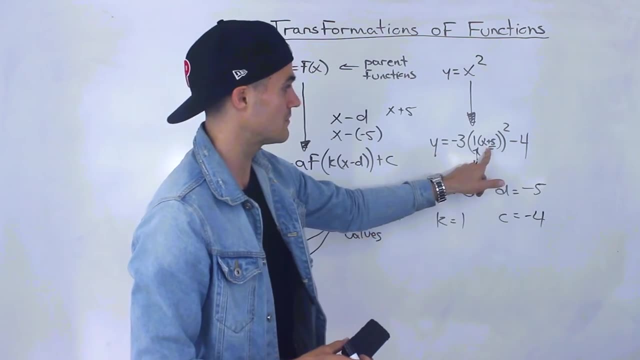 this. You won't have to rewrite it As time goes on. you'll just know you'll be used to it. but that's why this k and d value can be tricky, because the d value is always the opposite sign of whatever's here. and then this k value sometimes you have to factor it out in order. 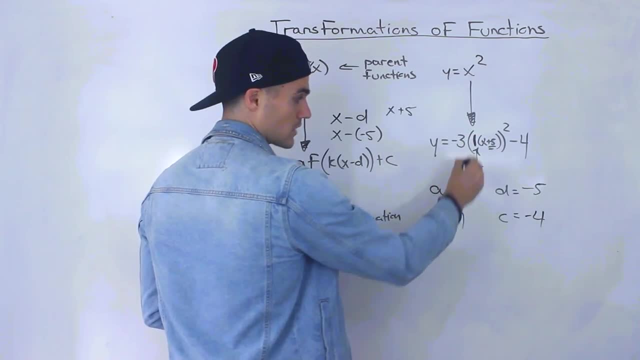 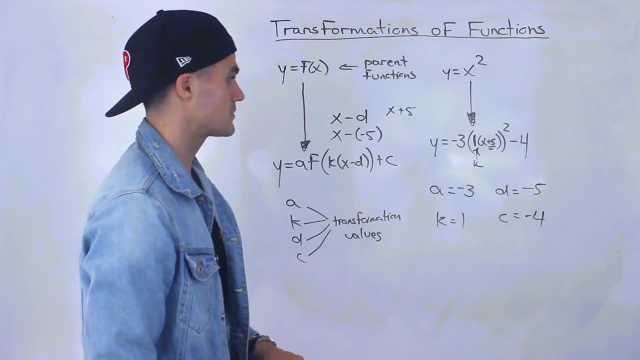 to get that k value. Sometimes it's not even going to be the opposite sign of whatever's here, which would end up being a one. Sometimes it could be negative, right? So these two can end up being a little bit tricky sometimes, but we're going to do a bunch of examples where getting 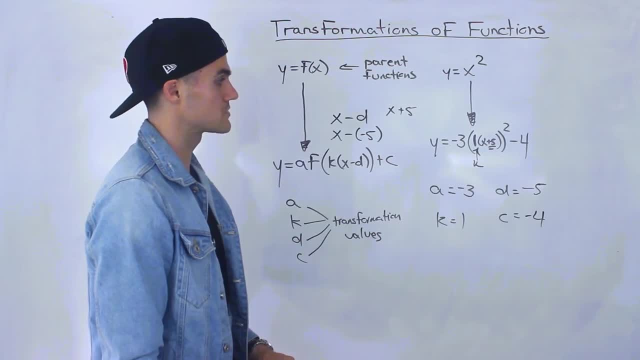 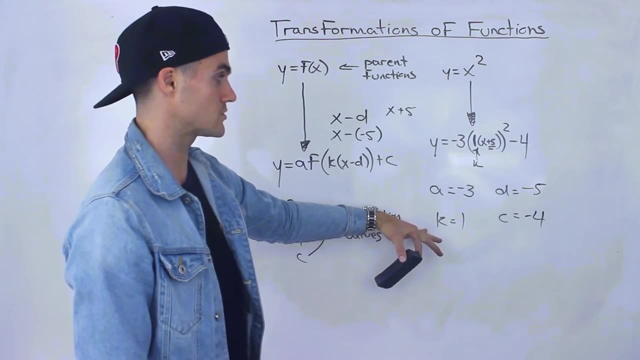 these is going to be like second nature for you after you go through the videos, right? So that's an example of taking a parent function, transforming it. Those are the transformation values. Another example is: let's say we take maybe the parent function square root of x. 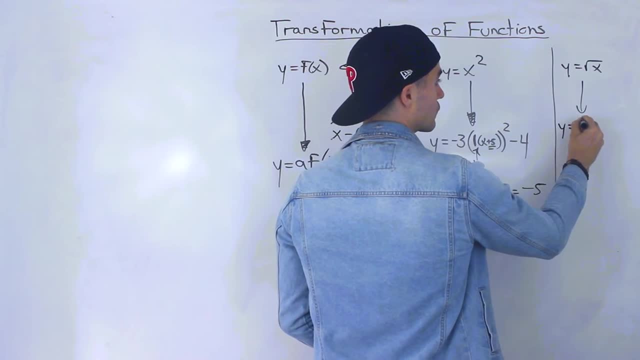 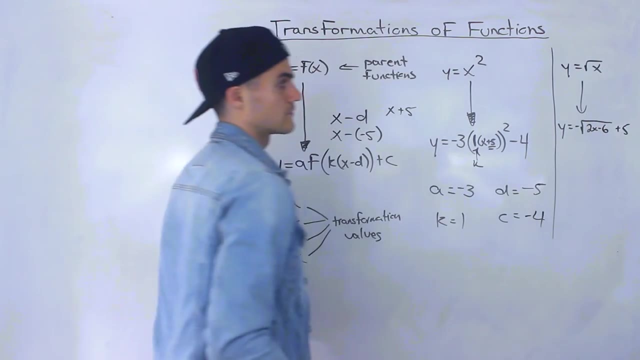 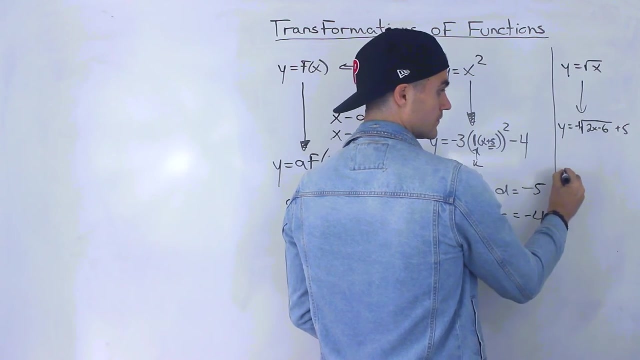 Let's transform it. Let's transform it to: y equals negative root. let's say: 2x minus 6 plus 5, okay, So what would happen here? Well, notice that the a value is negative. 1, right, If there's like just a negative. 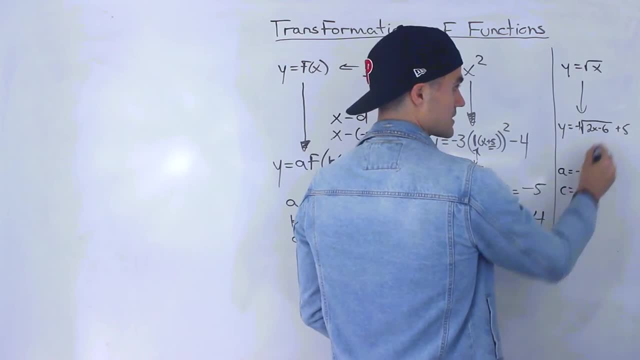 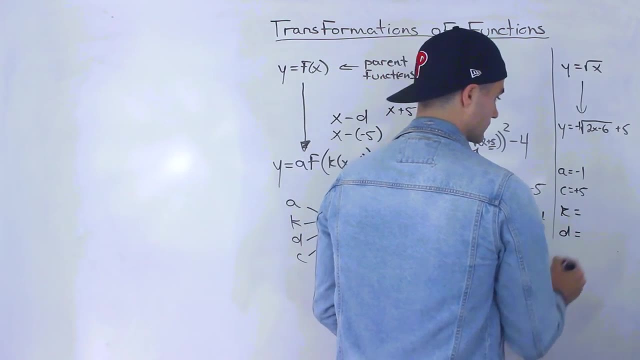 there it's like a negative 1. in front, The c value is this: outside, here It's positive 5, but what's the k value and d value going to be in this In this case? So notice that here, in this general transformation format, the x always has to be by. 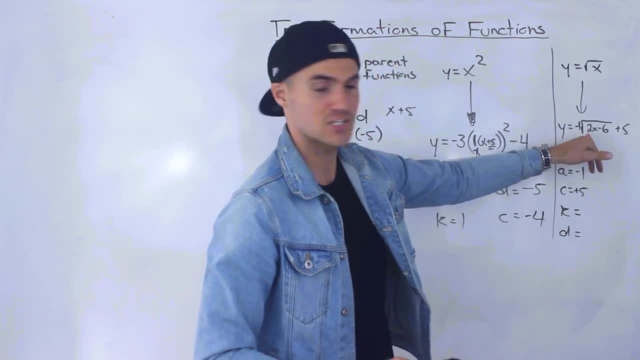 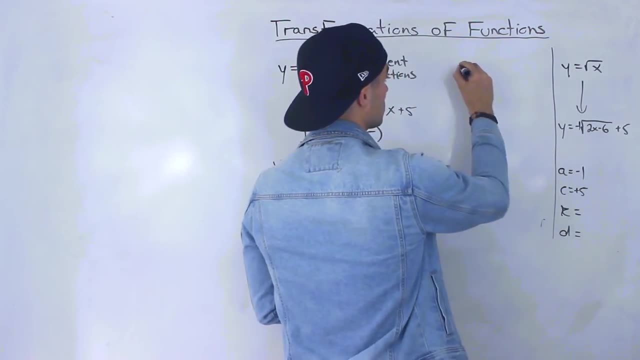 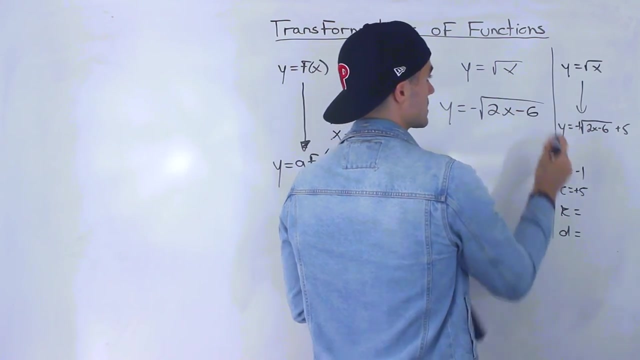 itself And notice that here the x isn't by itself, It has this 2 attached. So what we actually have to do, you know what? I'm going to: take this, rewrite it here, just to give myself some room, just so you can see it clearly. So we got: y equals negative root 2x minus 6, and then we got: 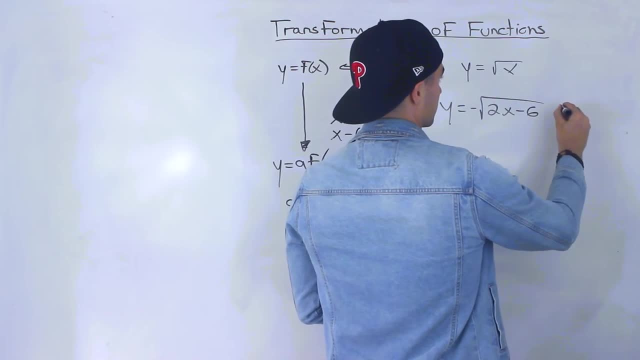 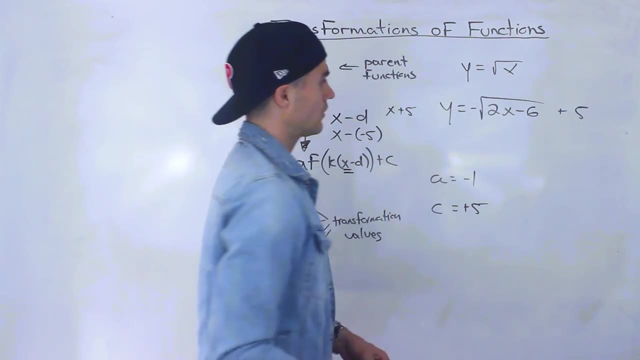 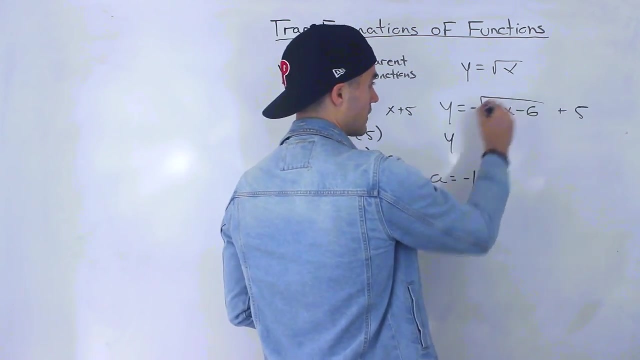 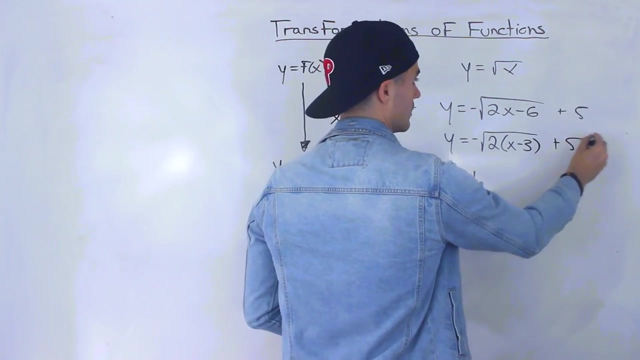 plus 5.. What we got to do is, in order for that k value to be by itself, in order for the x value also to be by itself, we need to factor within this over here. So we'll have 2 bracket x minus 3.. And now notice. 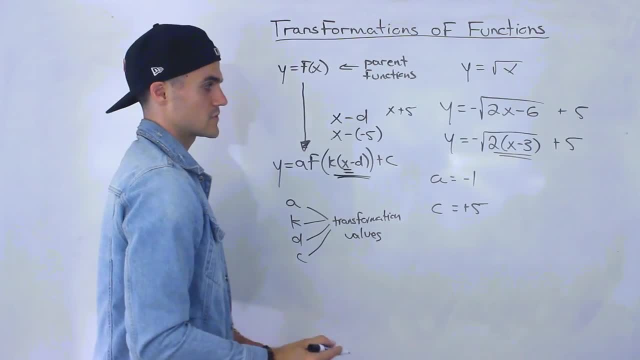 that this is in this format. So that's another reason why getting that k value and getting that d value is going to be by itself. So we're going to have to factor within this over here. So we'll have 2 bracket x minus 3.. So we're going to have 2 bracket x minus 3.. So what we're going to do is we're 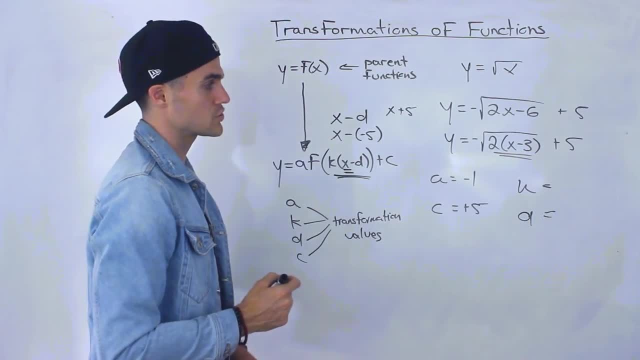 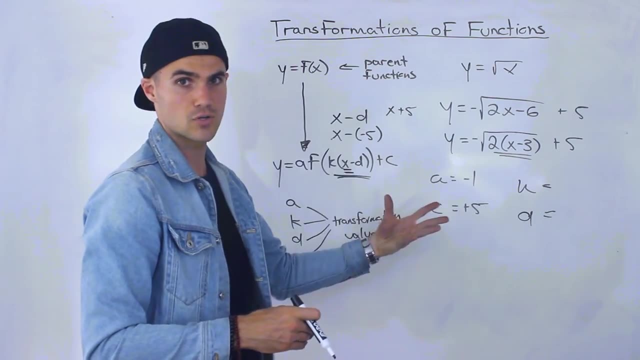 going to do a little bit of preliminary work And again we're going to run into a bunch of examples where we're going to be doing this. So don't worry if you're a little confused about what's going on here. As the videos go on, everything will sort of come together. So now that it's in this format, 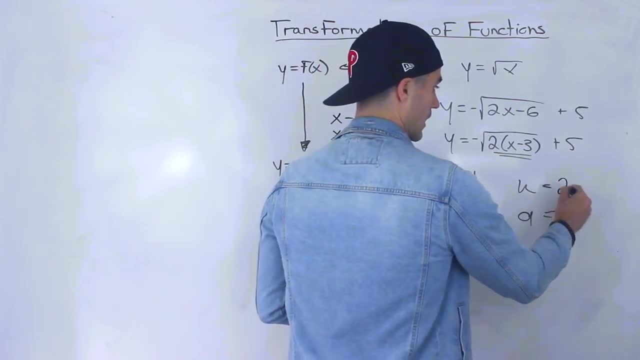 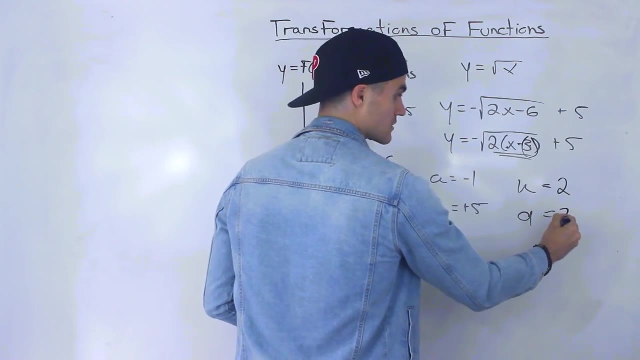 we could tell the k value is 2. And then the d value is what We got: x minus d, x minus 3.. So the d value is positive 3. it's the opposite sign of negative three right. so for something like this, these would be the. 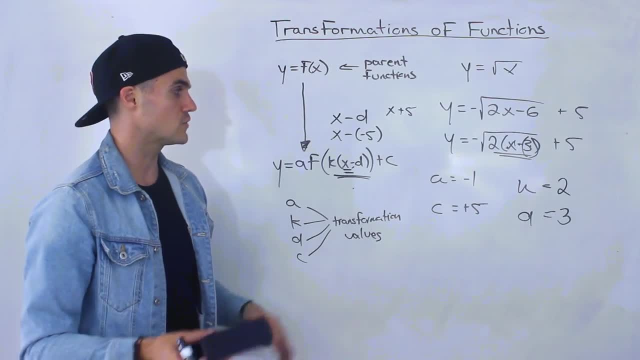 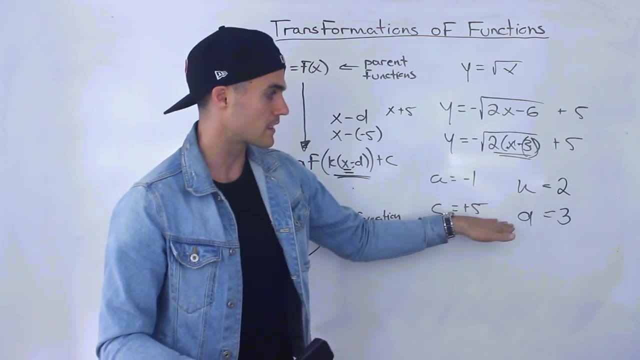 transformation values, right? so just wanted to give you a heads up of what's going to be going on, and actually, in the next couple of videos, what we're going to be doing is going through each of these letters in more detail and describing, depending on what value that letter takes, that transformation. 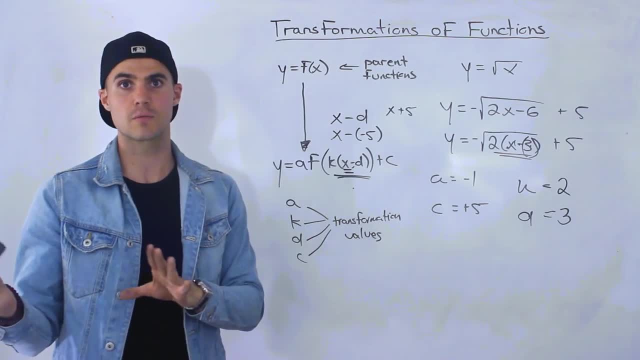 value takes what the actual graphical transformation is going to be, how it's going to look like on a graph.